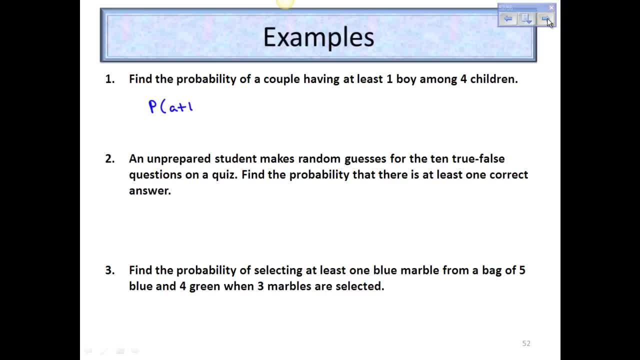 So the probability of at least one boy is equal to one, minus the probability of no boys. Let's decide. is this independent or dependent? Does the fact that you have a boy for one child affect the probability of having a boy for your next child? 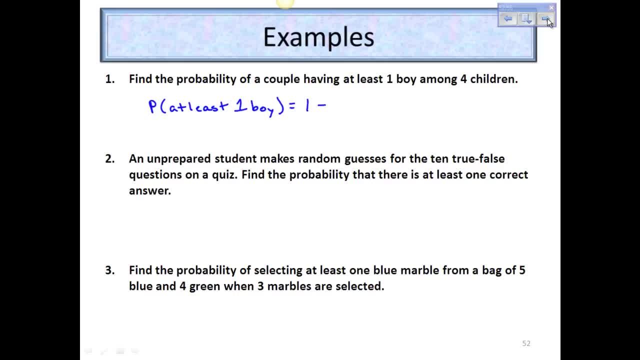 No, So these are independent trials- The probability of not having a boy- remember, we need the probability of none, So the probability of not having a boy in one trial, And then we're going to take that, And then we're going to take that probability and raise it to the number of trials. 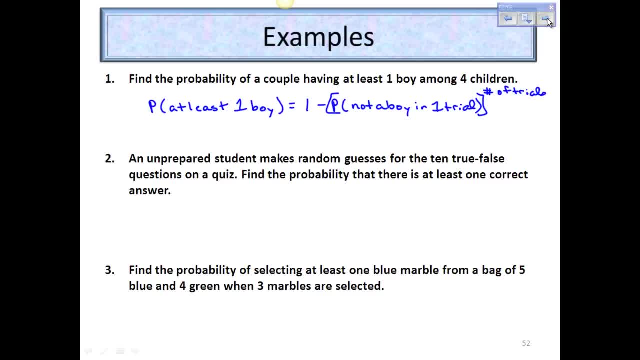 And in this case our number of trials are the number of children. So if you don't have a boy, you have a girl. so the probability of not a boy in one trial is still one-half. Raise that to four, So one minus one-half to the fourth is .938.. 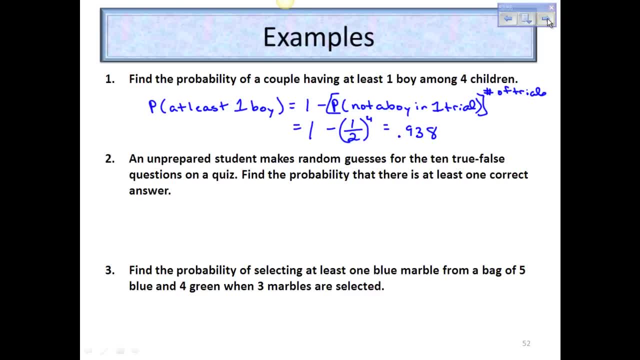 Example two: An unprepared student makes random guesses for the ten true-false questions on the quiz. Find the probability that there is at least one correct answer. So let's ask ourselves: are these independent? The fact that you answer correctly on one, does that affect the probability that you answer correctly on another? 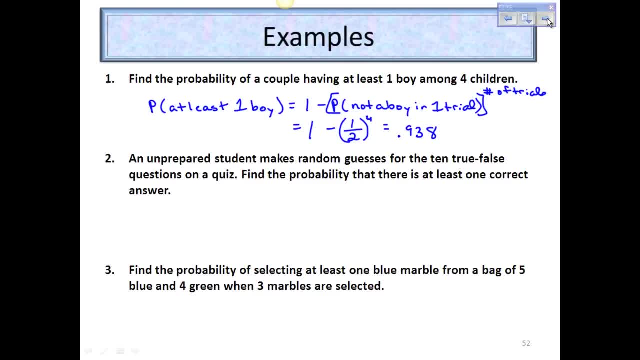 No, These are true-false questions. So answering incorrectly and correctly, does that affect the probability that you answer correctly on another? Absolutely, You have 50-50 chance, right? So the probability is one-half that you do not answer correctly. 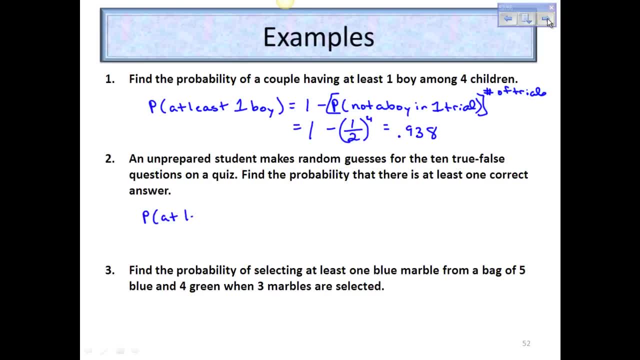 So the probability of at least one is equal to one minus the probability of none. Since these are independent and the probability that you don't answer correctly is one-half, we can take Find the probability of none by doing one-half raised to the tenth.